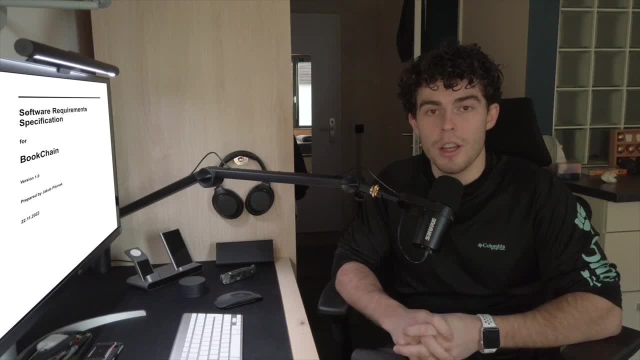 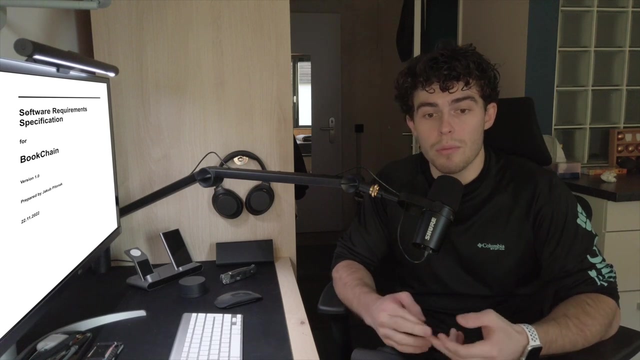 and I'll try to explain it in more simple terms. So an SRS document is this blueprint which is super detailed. It's kind of your wish list for your software, of what you wanted to do. You can think of this as this: as I said, a wish list which is super detailed and super organized And it goes from all your functional requirements, which could be how your software runs, all the way to your non functional requirements, which are 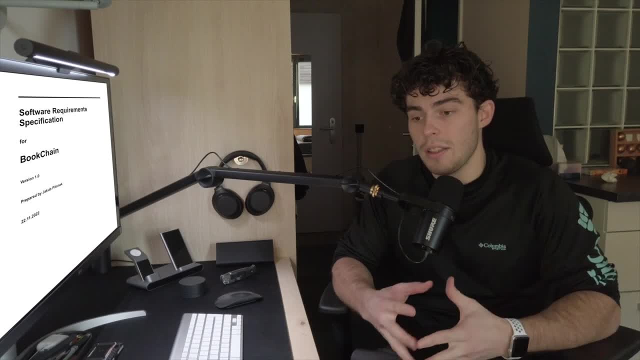 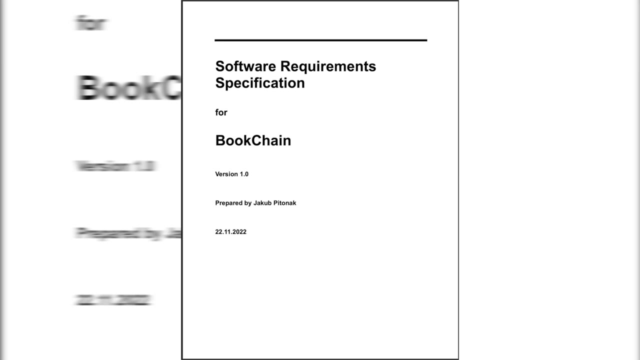 how secure it should be, how fast it should run, and terms like that. So now that you know kind of what an SRS document is, let's look at how I made mine. So all right, so me and my friend Adam, we had this idea for the software in mind for a while And and I thought that SRS document would be a great opportunity to really create a detailed 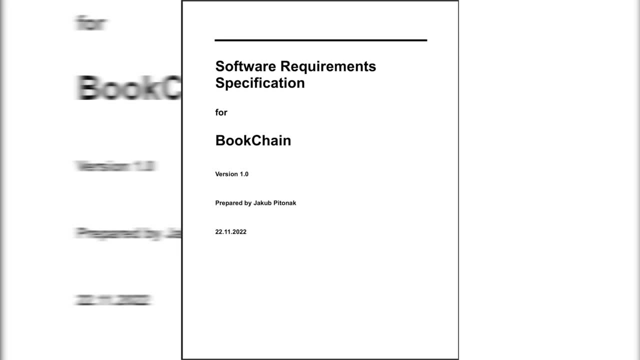 INSPRETATION blueprint for it. So the project will be called Ewives Business, which retains data on all the. So the project called book chain And it is a project called software that aims to bring digital ownership to the world of online book articles and says: 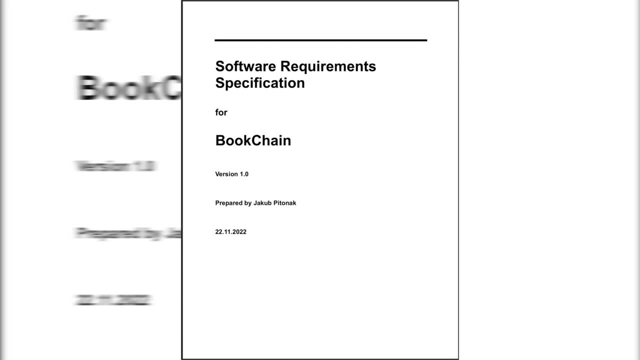 So the project quiet publications s and publications. with the implementation of book chain technology, encrypted wallets, users would be able to own their digital assets and sell them if they no longer need them. This would give the users your option to sell the digital books just like they wouldn't physical copies, because release data of all digital assets. 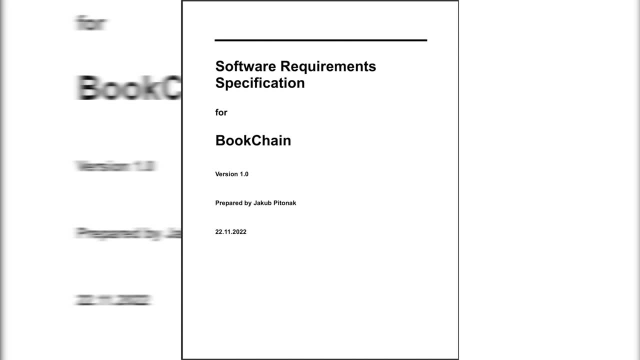 benefits. interest wouldfounder could connect to tools and market. right now, after you purchase a digital book online, you most likely will just get the pdf and there's not really a secondary use to that. so now to the publishers and writers. who would be? who would be? 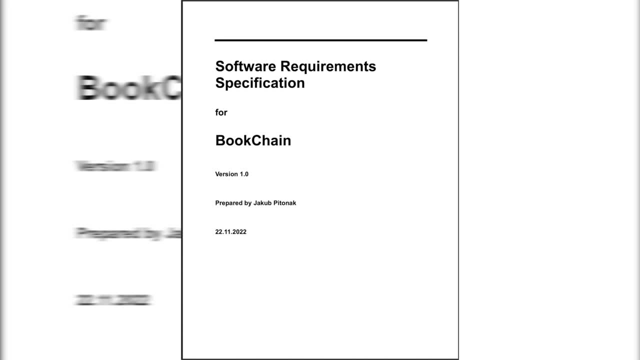 also benefiting from the book chain, as they would be able to publish their work there and receive their payments for initial sales with a royalty paid for every secondary sale. book chain aims to replace the current system of purchasing online articles with the added feature of being able to. 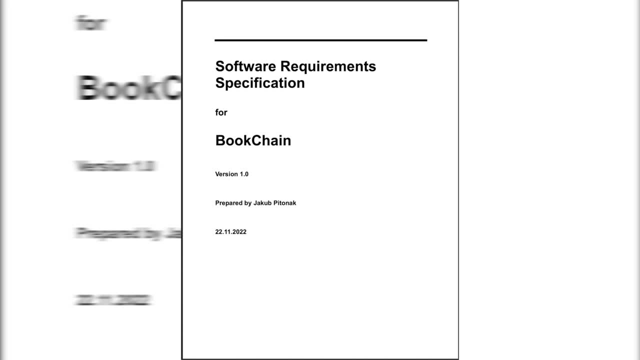 sell them back to the marketplace. this would allow the users not only to sell their items, but also accumulate value in their collection, with limited releases and special edition, for example. all right, so that is this description of the project, and now we can go through the actual srs document and see how i sectioned everything so, as every good document starts with uh, with the 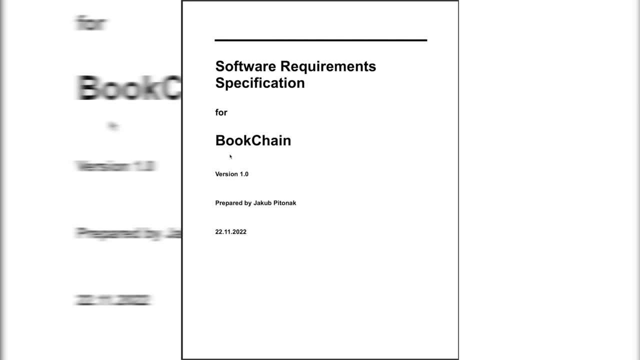 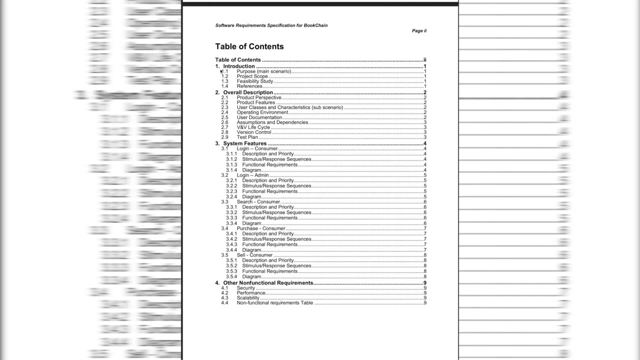 first front page with the what the document is about, who published and who prepared it- you. so we started with the table of contents, where we can see that i first started with introduction, then the overall description, continue with system features and then finish that with non-functional requirements. so since i was working independently on this project, the first step was to define the 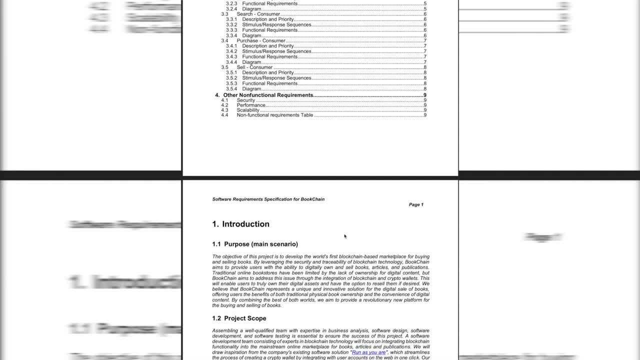 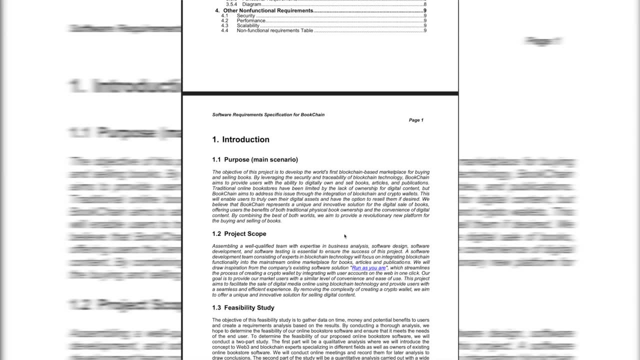 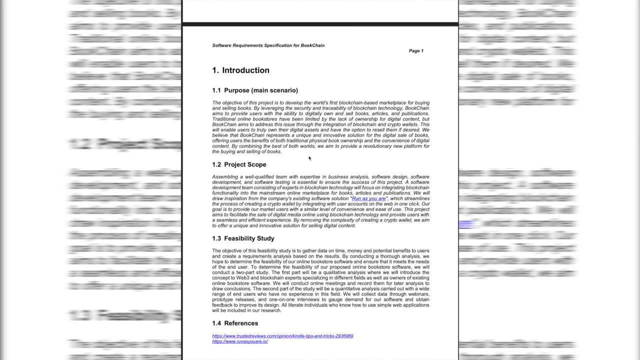 requirements myself, based on my own image on the software and the needs for the user. to deal with this, i did some research on similar software products and industry standards to get sense of what was possible and expected. so here i started with the introduction and some general purpose. 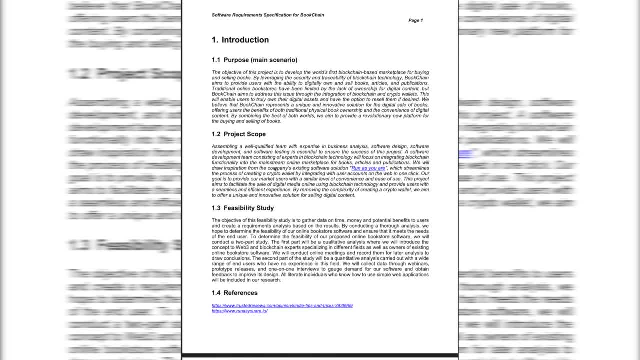 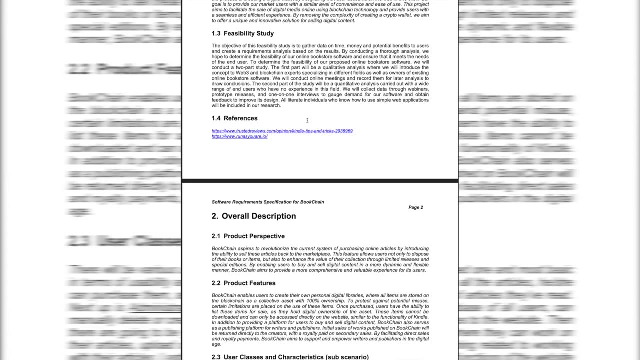 then we continue with the project scope. this was a similar software that is running, run as you are, shout out to fun as you are. they're really awesome software. and then, after i had all of this prepared an introduction, i did the overall description okay, so this is just more going into, more into details. 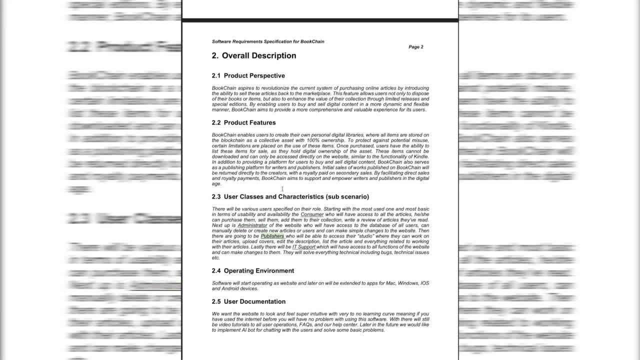 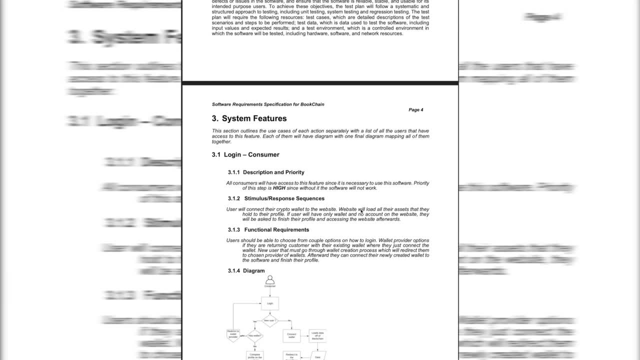 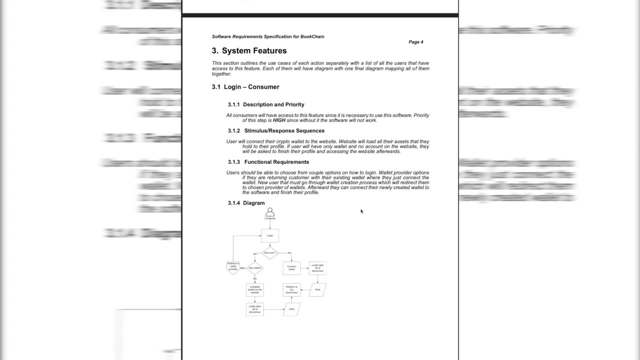 creating some of the users that would be using the apps, and then we continued to system features. So, continuing down here, I wrote a detailed description of each requirement, including any constraints or assumptions that were relevant, made sure to be specific and clear as possible. 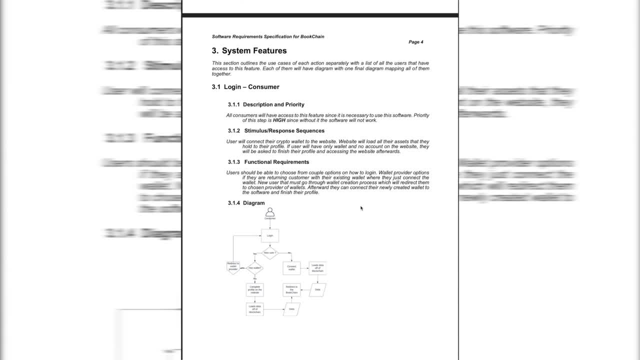 and this would help to prevent any misunderstandings. during the development process, I also included examples and scenarios to help illustrate how each requirement would be used in the real world. This was especially important for requirements that might not be immediately obvious or intuitive. After I had written the description for all the requirements, I reviewed the SRS document. 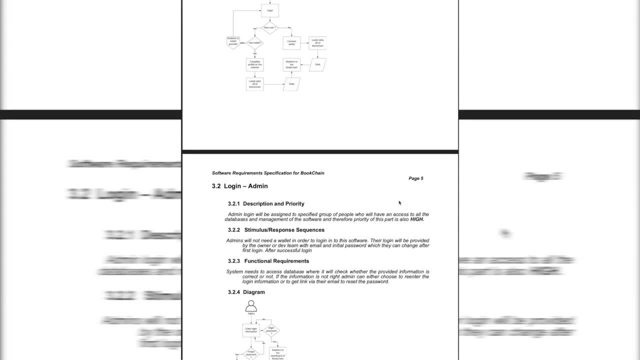 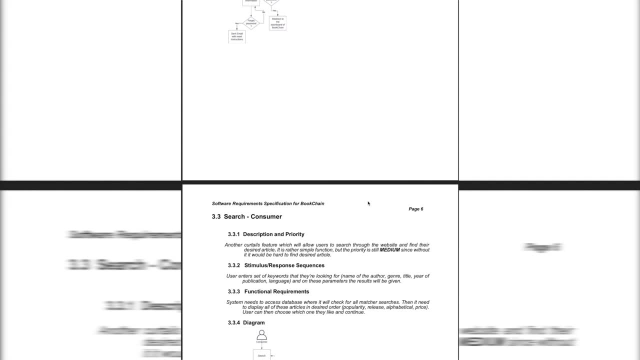 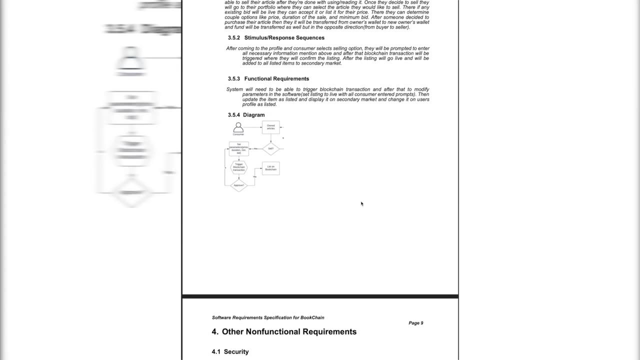 myself and made any necessary revisions. I also showed the SRS document to friends or colleagues who are familiar with the software development to get their feedback and ensure that the document is good. It was clear and comprehensive. Then, lastly, on the page, I think, of TIAT 9, I've included all non-functional requirements. 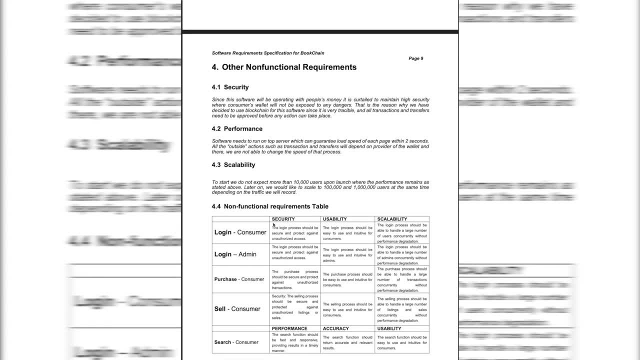 that were needed for this software, as is security, performance, scalability or usability, accuracy, And here I listed all the again constraints or some limitations that the development team would need to look out for while developing the software. So, finally, I had everything done. 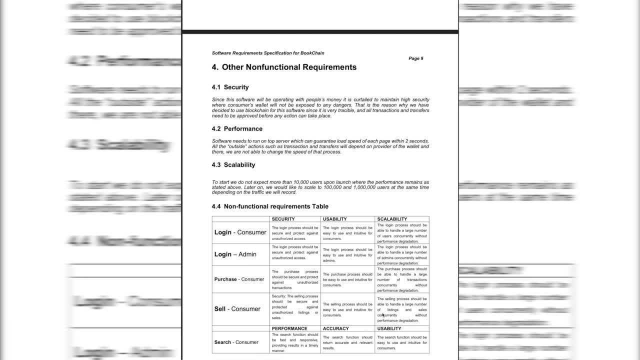 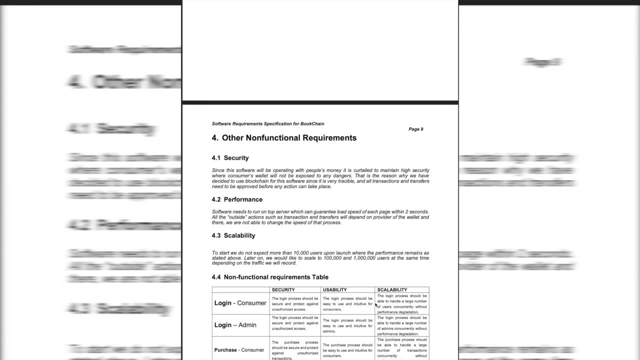 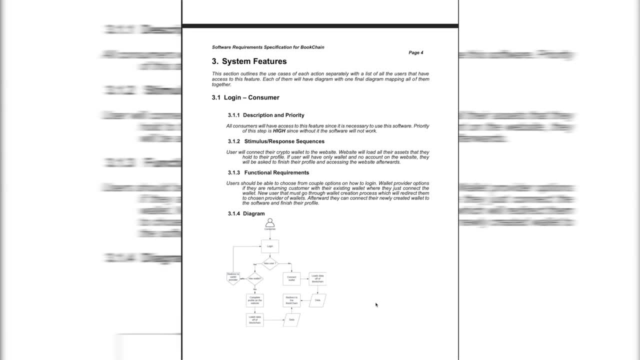 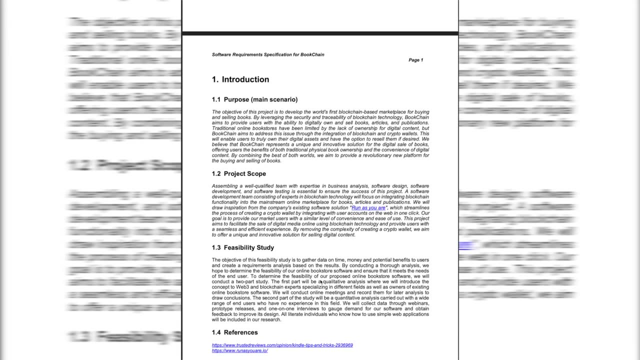 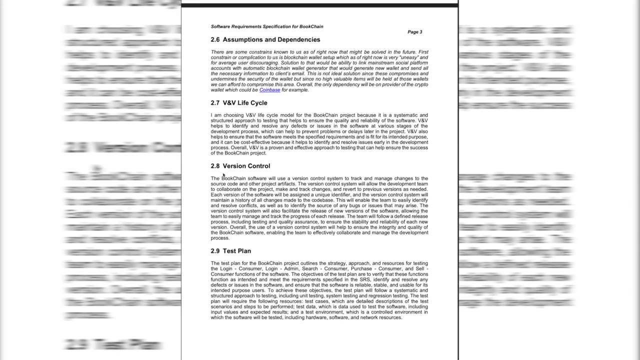 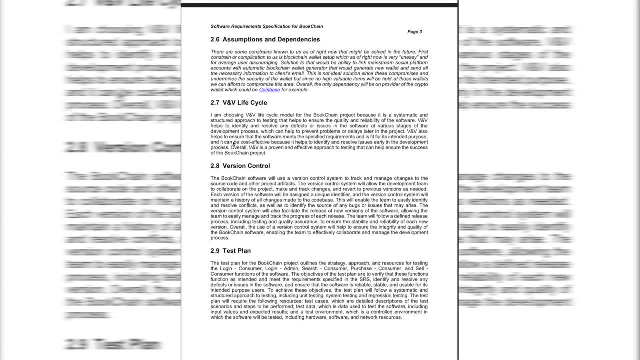 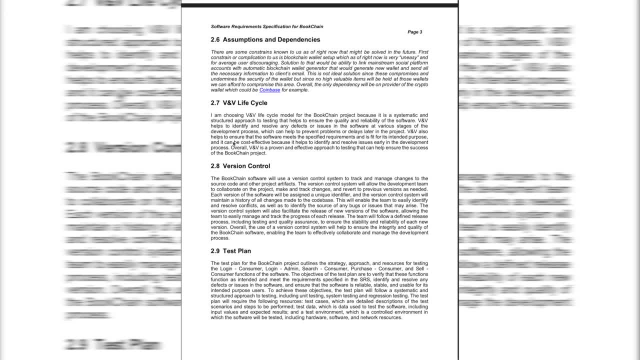 success of the project if I will ever try to implement it. So I hope this video was helpful and gives you some insight into process of creating an SRS document. I would really appreciate your thumbs up or comment if you have any questions, And thanks for watching and I hope to see you in the next video.